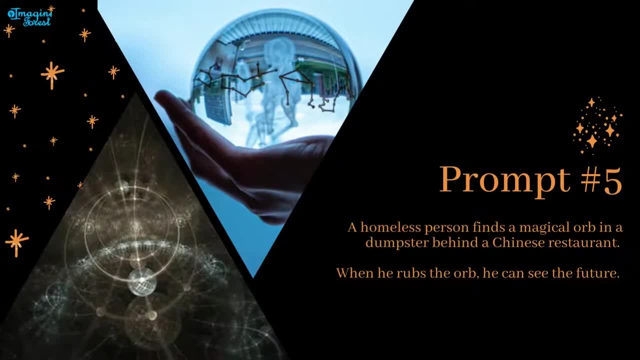 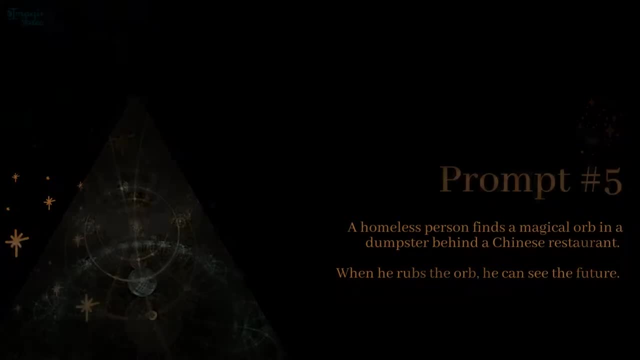 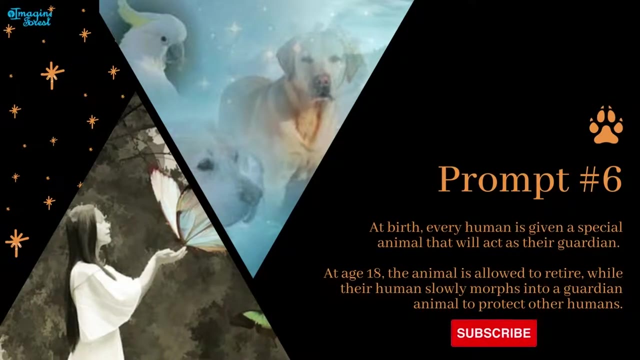 When he rubs the orb, he can see the future Number six. At birth, every human is given a special animal that will act as their guardian. At age 18, the animal is allowed to retire while their human slowly morphs into a new animal. 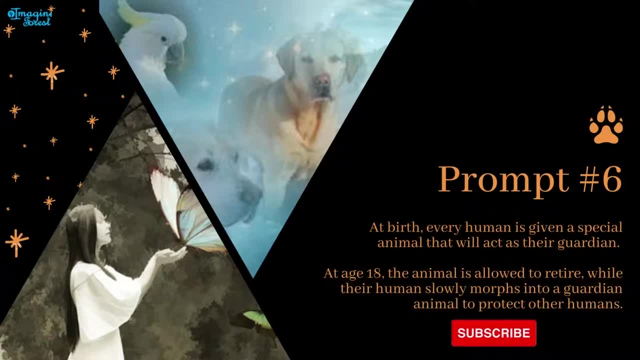 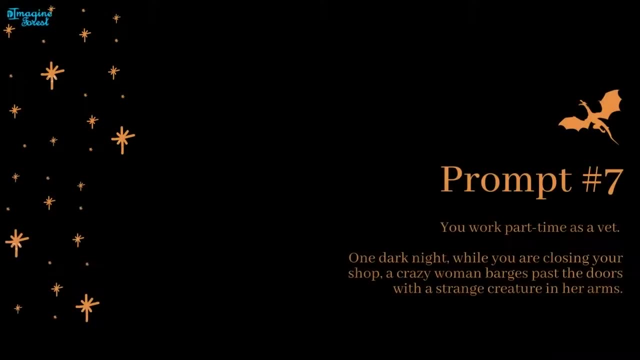 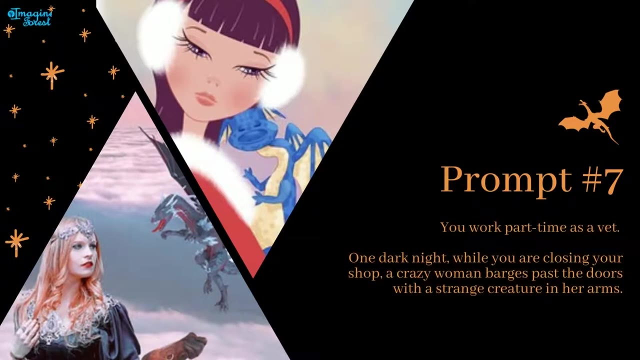 Number five: A ghost is found in a dumpster behind a Chinese restaurant. When he rubs the orb, he can see the future. Any chance for the ghost to get back again? Number seven: You work part time as a vet. One dark night, while you are closing your shop, a crazy woman barges past the doors with a strange creature in her arms. 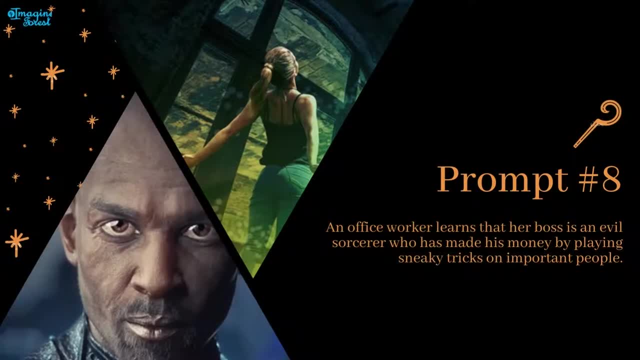 Number eight: An office worker learns that her boss is an evil sorcerer who has made him shades in action money by playing sneaky tricks on important people. number nine: the legend goes that there is a secret world that you can only access through a magical. 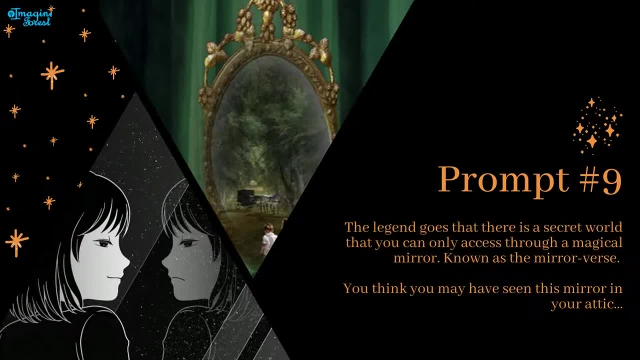 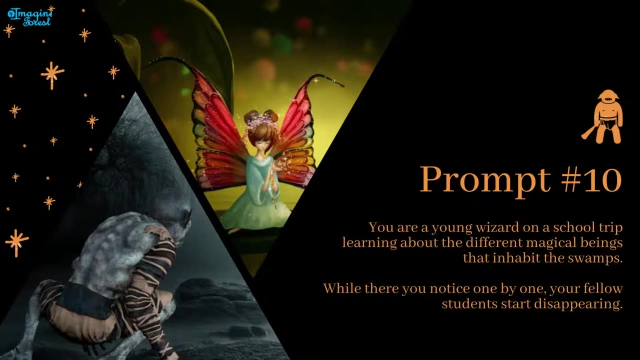 mirror, known as the mirror verse. you think you may have seen this mirror in your attic number 10. you are a young wizard on a school trip learning about the different magical beings that inhabit the swamps. while there, you notice one by one your fellow students start disappearing. 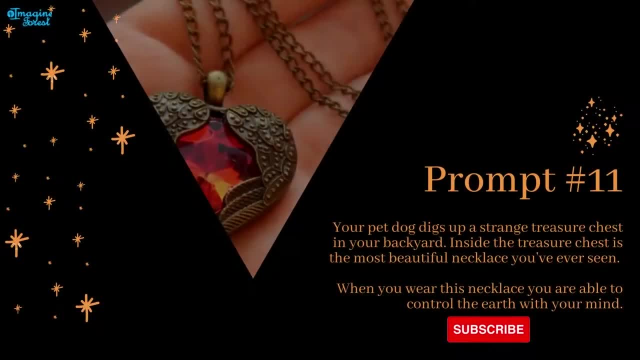 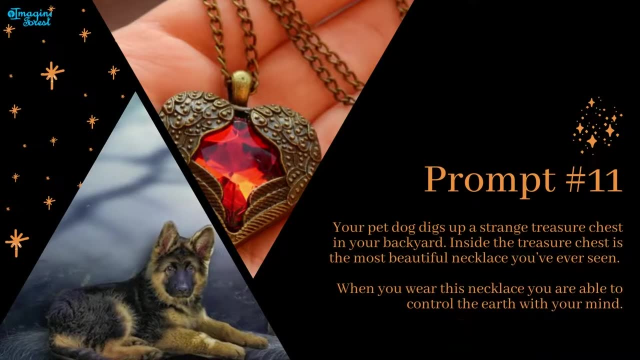 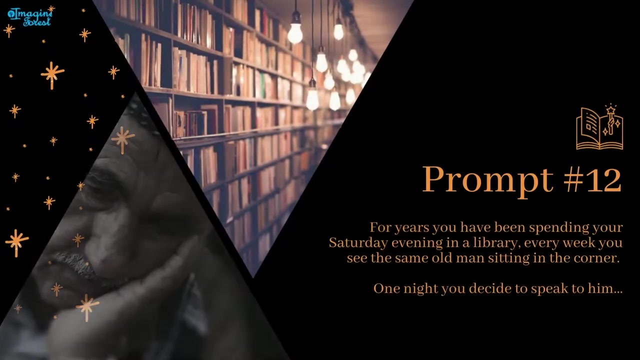 number 11: your pet dog digs up a strange treasure chest in your backyard. inside the treasure chest is the most beautiful necklace you've ever seen. when you wear this necklace, you are able to control the earth with your mind. number 12: for years you have been spending your Saturday evening in the 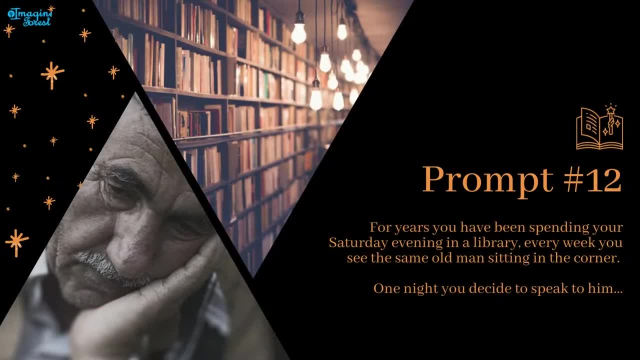 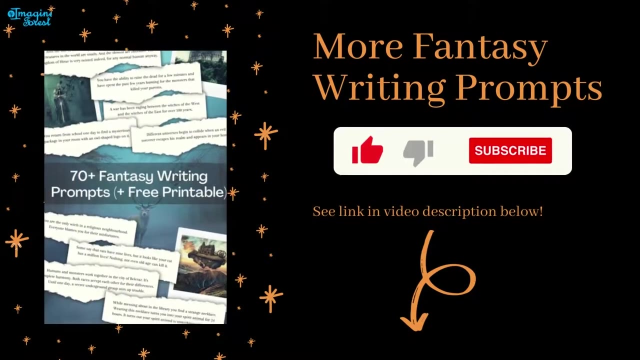 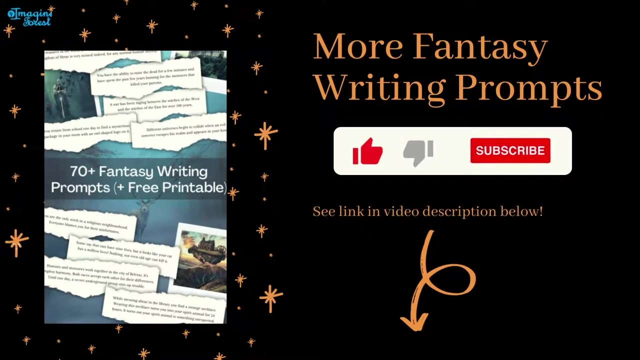 library. every week you see the same old man sitting in the corner. one night you decide to speak to him for more magical fantasy, writing prompts and an idea generator. check out the link in the video description below. that's all from us today. let us know in the comments below if you were able to complete all 12 fantasy.